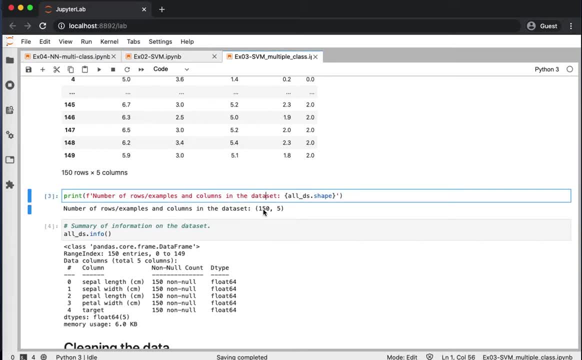 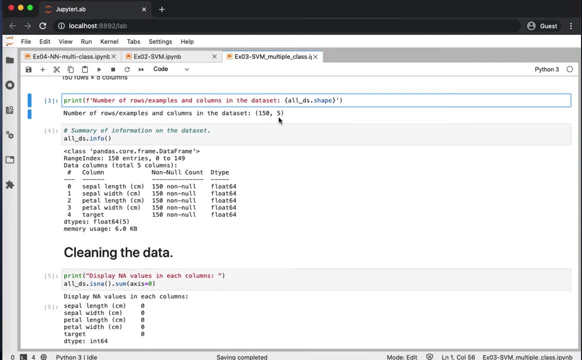 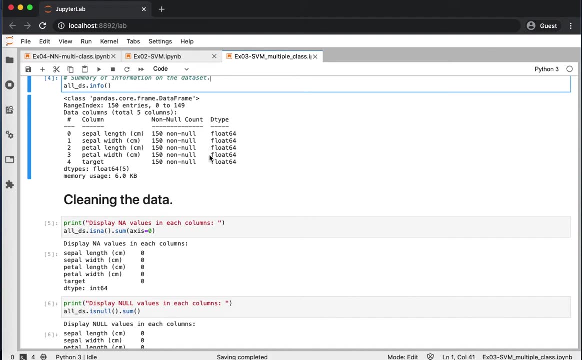 Then we have 150 examples. when I plotted the or, I tried to show the shape of the overall dataset. it's 150 examples and five columns. Let's see the data type of each column. so it looks like all of them are float, which is good, so they are ready for us to start working on them. We checked for. 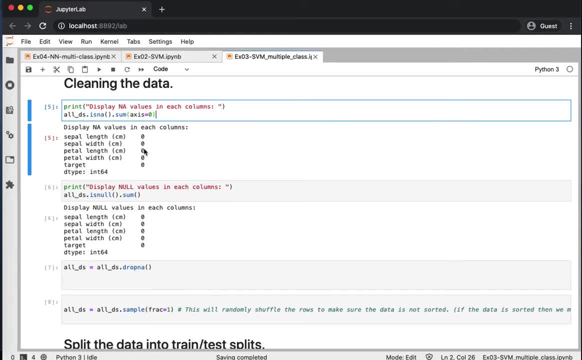 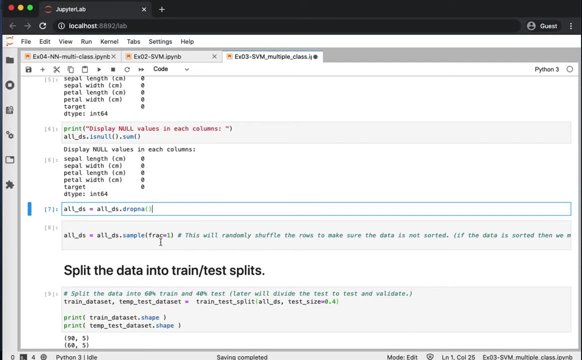 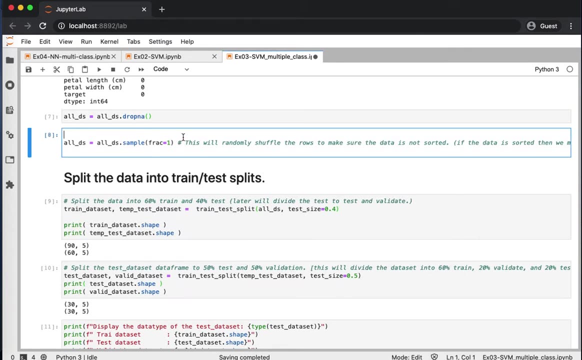 missing data points and to clean this data. it looks like we do not have any missing data points. If we do have, we can drop them or impute them. I like to shuffle the data and reorganize it randomly. so the data is reorganized randomly, so it's not ordered in a certain way. 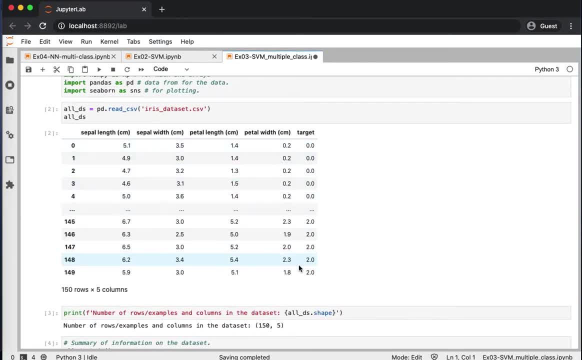 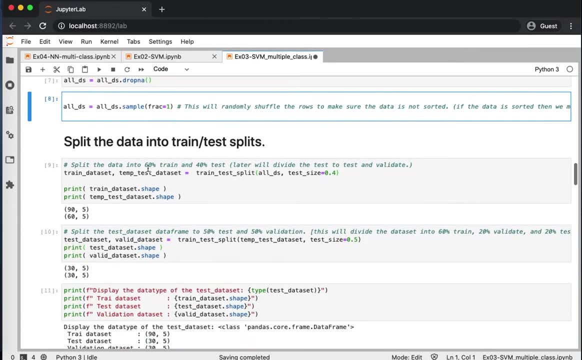 So if you look at the beginning, when we started the data, it looks like it was sorted based on the target, so now it should be shuffled and reorganized randomly. Let's split our data and I will use the same convention that I use always, which is 60 percent. 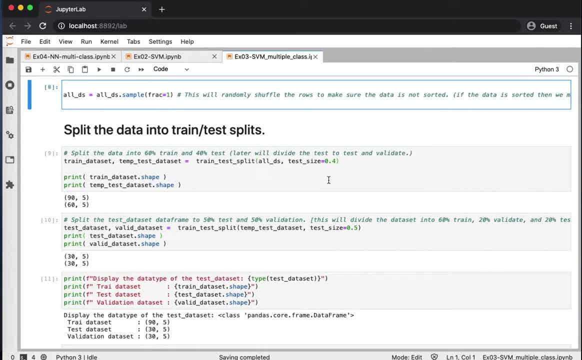 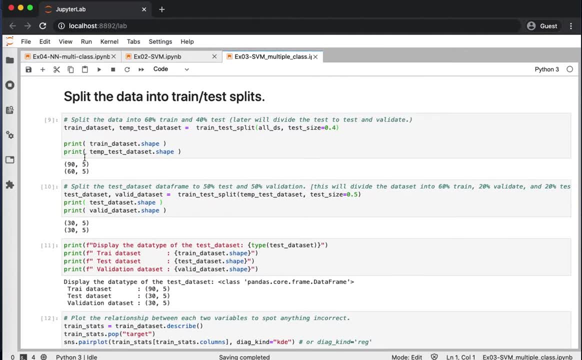 and 40 percent: 60 for test, for training and 40 for validation, cross validation and testing. So therefore, we divided the data into 90 and 60. The 60 is split into three and a 30 and 30, which one which is one for cross validation and the other one is for testing. 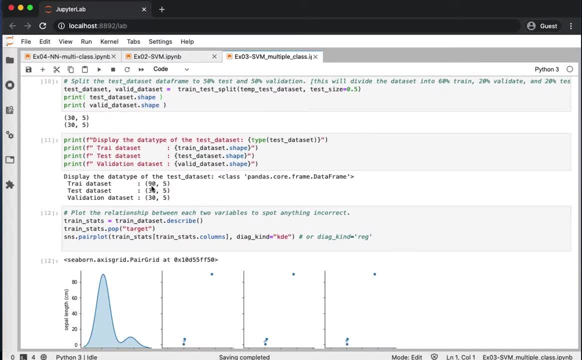 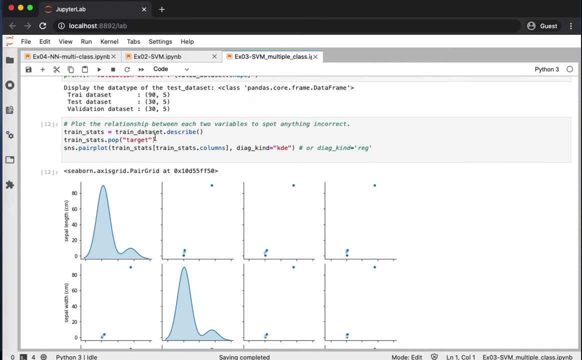 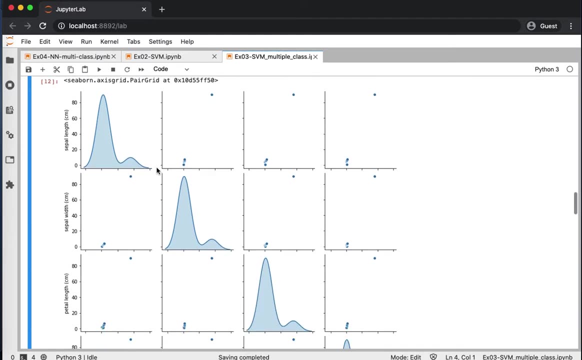 Now let's plot or display the shape of our data and the training is 90, test and cross validation are 30 each. Let's pop the, the remove the target or the class label and plot the data, just trying to see the relationship between each pair of variables. 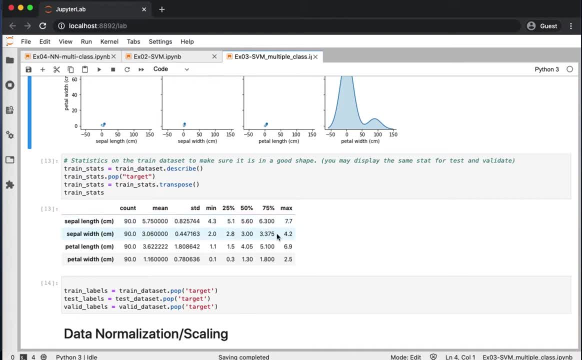 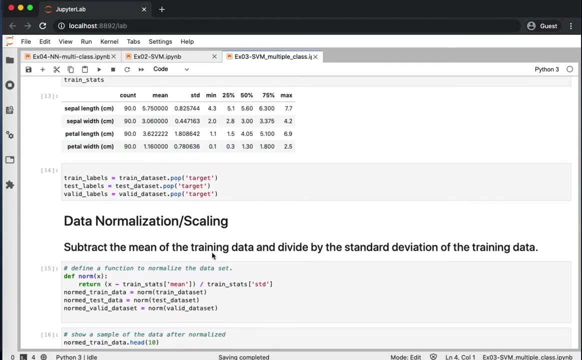 and then show the description so we can see the minimum and the maximum. This data set is in different ranges so therefore I need to scale it. We remove the target or the label of the or the actual label and we place them in three separate variables: one for training, testing and 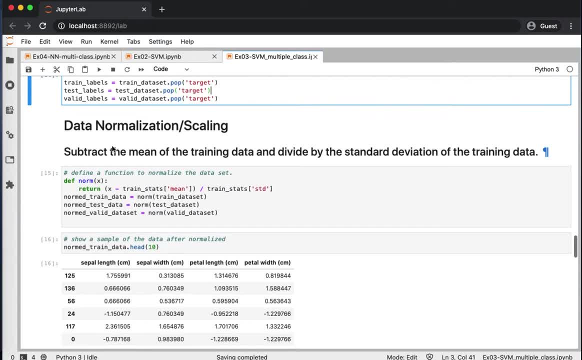 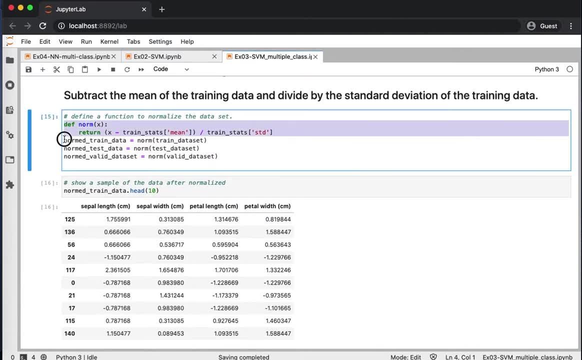 the last one is for cross validation. We normalized our data by subtracting the mean and dividing by standard deviation. We constructed a method in here for that, and then we call this method for training, testing and validation and then saved the results in three different new three variables. 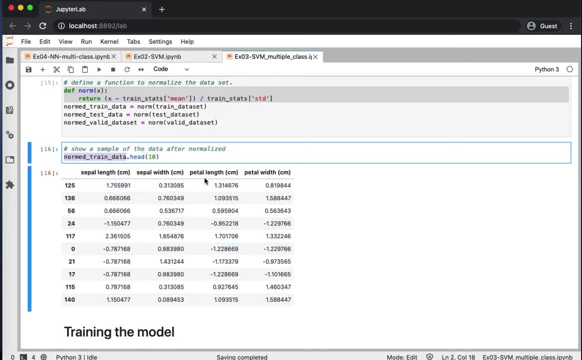 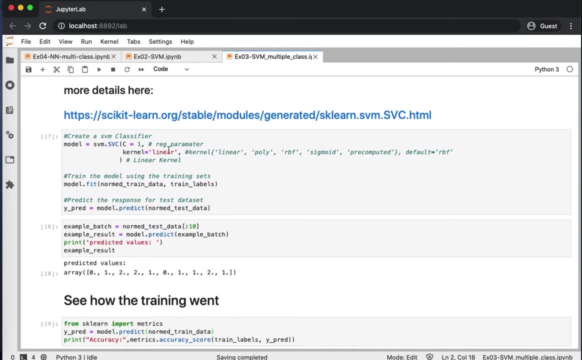 Then we displayed part of our data just to have a look at it and it looks like again it's shuffled, the indices are not sorted and the data is scaled and it looks within an acceptable ranges. Now we will use sklearn, and this is where you can find the package and more information about. 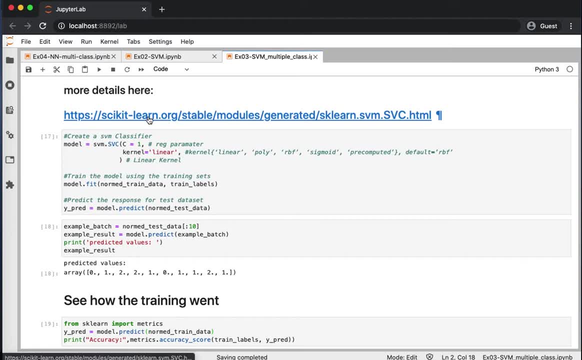 sklearn or scikit-learn about support vector machine from sklearn and And I will use or create SVM. and remember SVM is an object that we imported from a scalar in all the way on the top and then sv just to create the settings and the configuration. 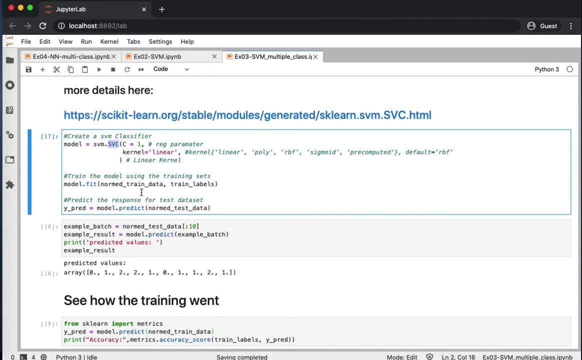 of the model. There are many parameters that you can play with for the support vector machine, But just for the sake of this video, in this class we will just focus on the C, which is the regularization term or the regularization parameter, as well as the kernel. 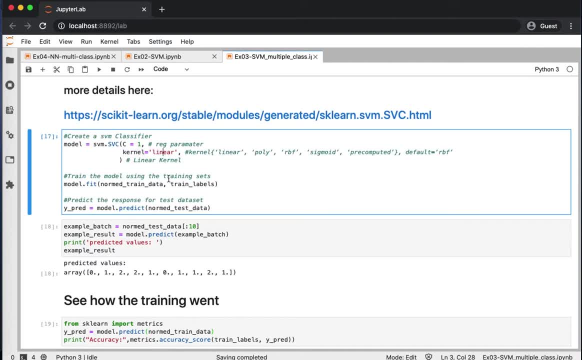 Initially we will use a linear kernel that's very similar to logistic regression. Then feel free to pick any of these other kernels and evaluate them. I fit the data as well as the labels, and then we try to predict the labels for the testing dataset or the validation dataset. 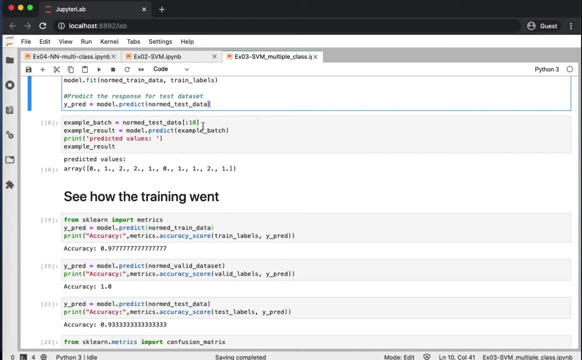 To fine tune the parameters. We also selected randomly, or we selected the last 10 examples from the test dataset and we try to label them and display the results. And it looks like the labels are from 0 to 2, as expected, three different labels. 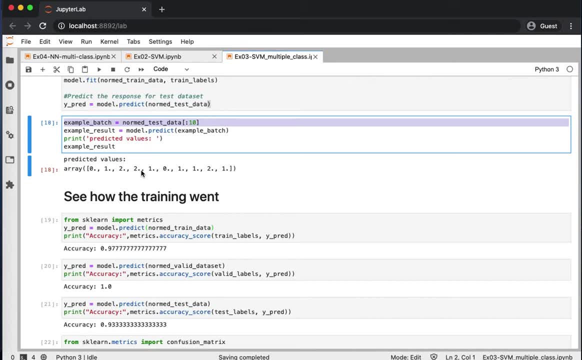 As you see in here, training a support vector machine as a binary classifier or multi-class classifier has no difference And in terms of the training, because the model will determine how many classes you have, So you do not need to have a special treatment for binary classifiers or multi-class classifiers.